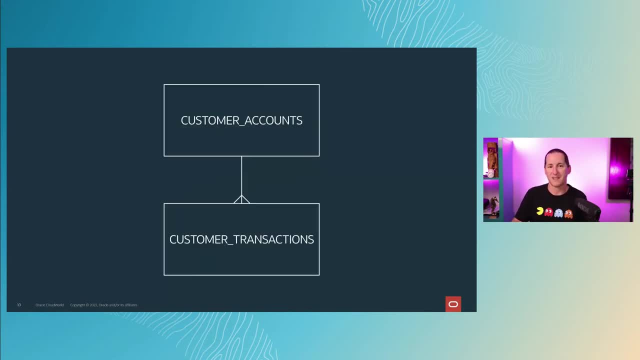 a real customer I worked with many years ago before I joined Oracle. This was a retail customer And, as you'd expect, the data model had customers with one row per customer plus a child table of transactions. New customers sign up And when they sign up, they're going to be able to. 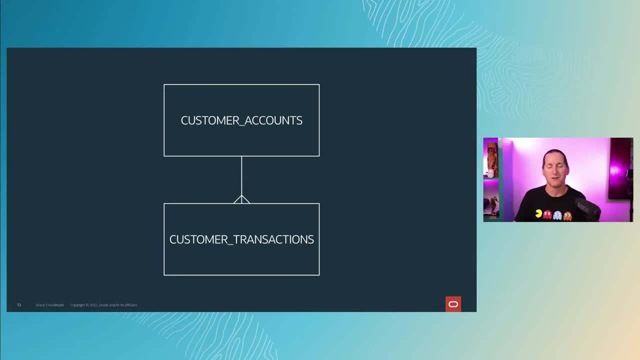 buy something, They add a row to the transaction table. I won't reveal too much more to preserve anonymity, but we had hundreds of millions of transactions every single year. A requirement came in from the business saying: give us a report of the most recent transaction date for. 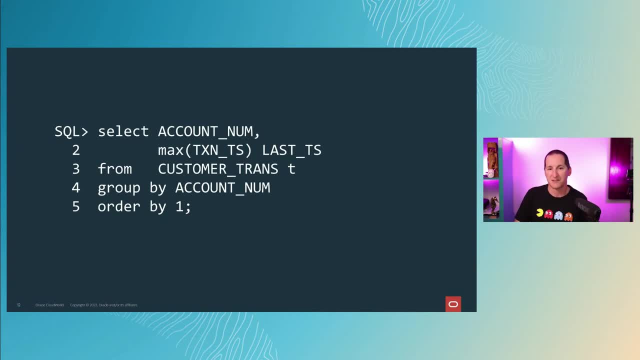 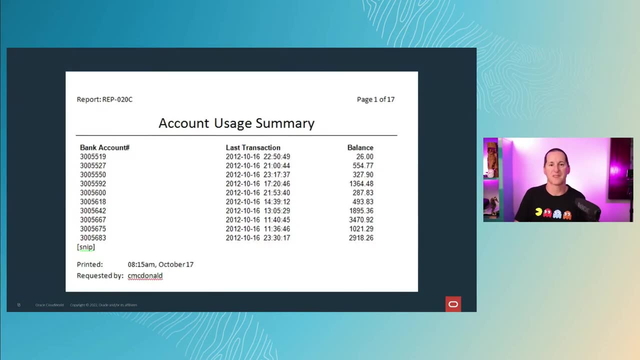 each customer. Now that's a very easy SQL statement to write. We simply do a max on the transaction timestamp from our customer transactions table and we group by the customer account. This gave us a report like the one you can see here: one row for each customer with the. 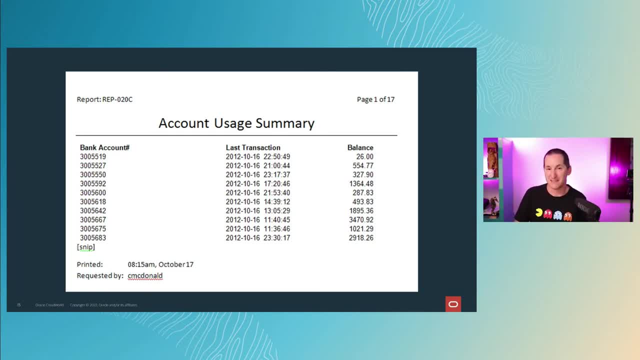 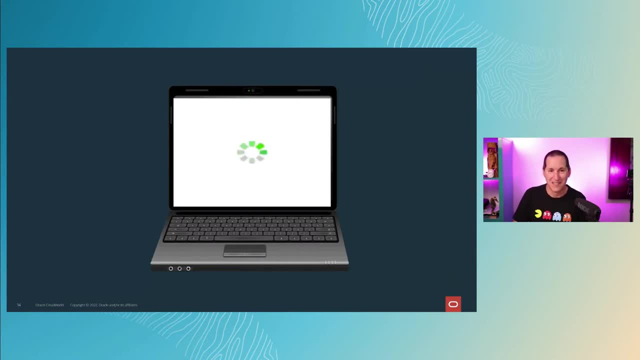 most recent transaction details. There's no problems with the complexity of that SQL statement, but there was a problem when we ran it And that problem was very simple. It's the famous hourglass. It took forever. It was fine in the early days, but as the volume of data grew it got slower and 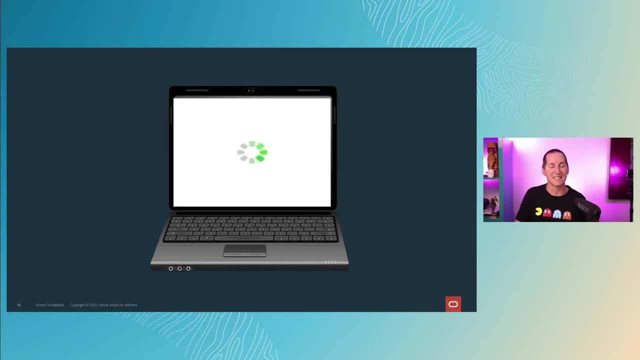 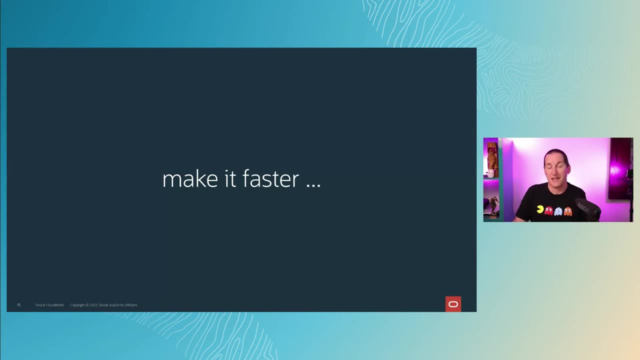 slower. Thus, eventually, the phone call that we all dread came in, and that's namely: please make it faster. We need this report every single day, And so began a series of attempts by us to tune this SQL. The first thing we tried is a time-honored technique, which I refer to as the Kiwi technique, and 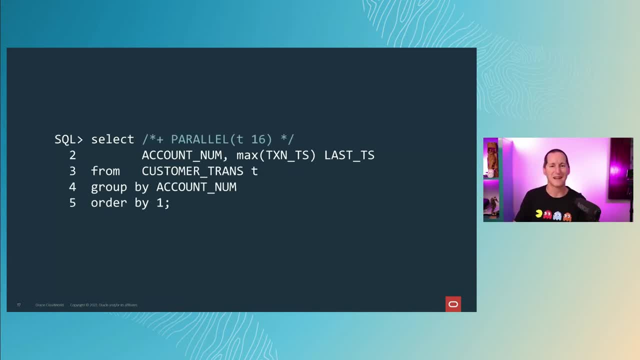 that is, kill it with iron. If something is slow, then just whack a parallel hint on it. grab a bigger slice of the server pie. This indeed did make the query faster, but the lights went dim in the server room. the IO subsystem got hammered and generally everything else in the application. 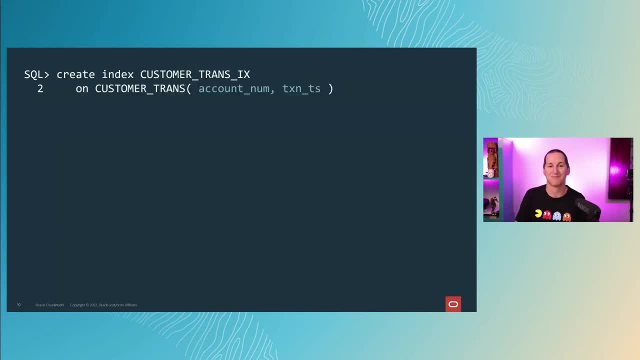 bogged down while we smashed the database server to get this report done. So then we tried adding an index to just the columns we needed to scan this query. In that way we could scan a thinner version of the table being just the index. That worked too, but 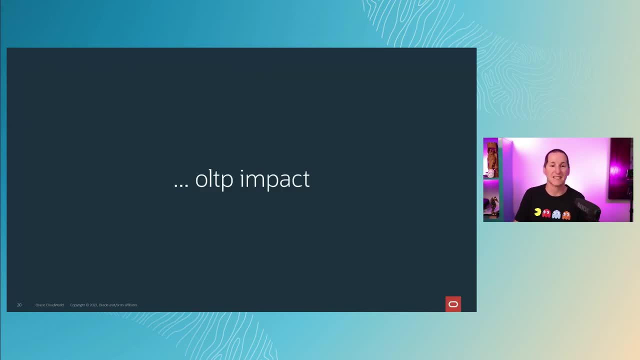 when you're dealing with high transaction volumes, like we were, every index has an overhead to the transaction response time. So we had a report that ran okay, but we added a performance penalty to every single transaction that we ever took from customers. So then we looked at partitioning the transaction table- Simply breaking a large table into smaller. 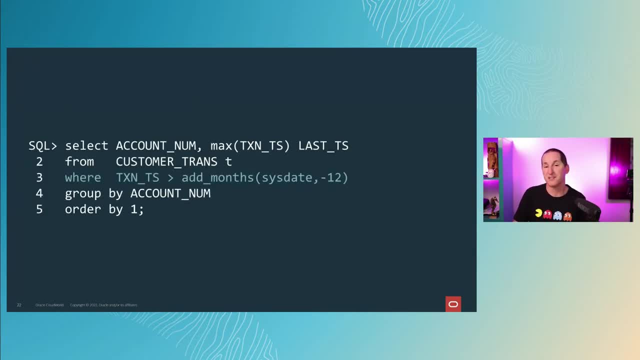 chunks does not by itself make queries faster, But we altered the report definition to show the last transaction only if that customer had had a transaction in the last 12 months. In that way we were scanning just the report last 12 months of. sorry, in that way we were scanning. 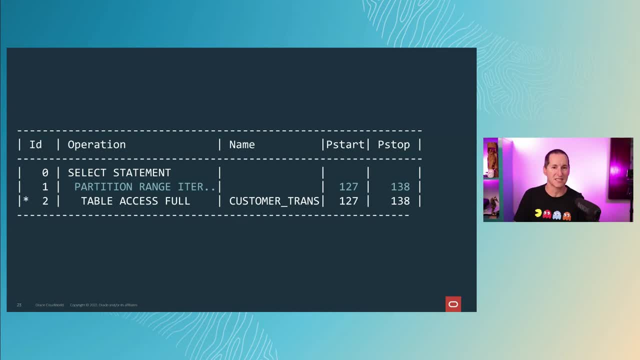 just the last 12 months of table data and hence only 12 partitions of the table got scanned, no matter how large the table got. That worked, but in doing so we had actually changed the function of the report. Now the report was somewhat vague when it came to customers who were not active. 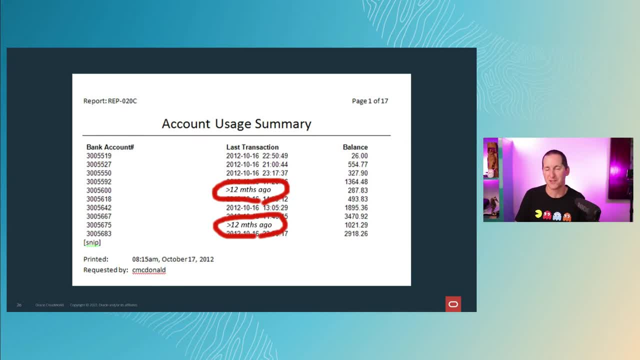 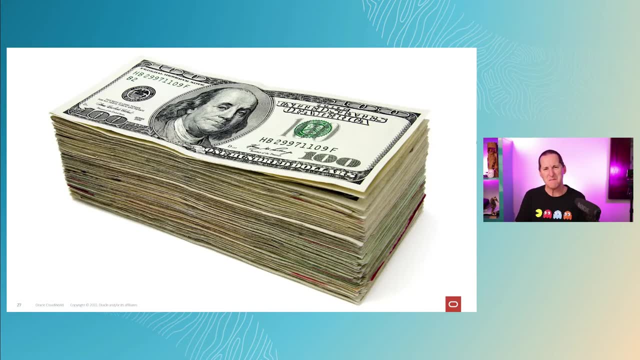 in the last year because we did not have the transaction details for them, We had reduced the quality of the report and we now had a petitioning license. to pay for More money for less functionality is never really a great sales pitch to your business. 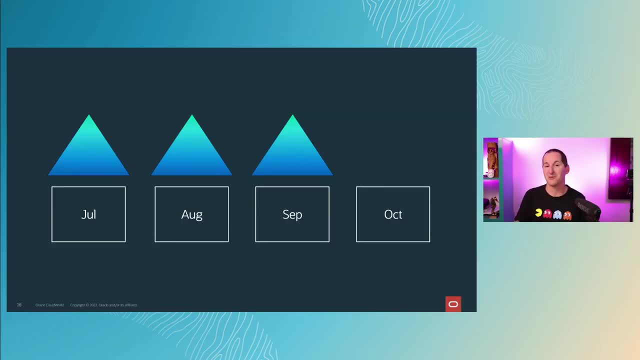 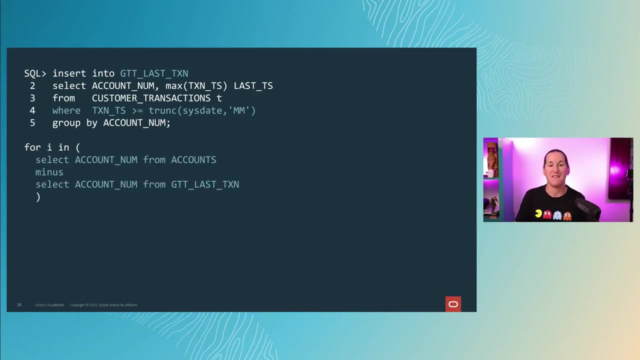 representatives. To overcome that, we tried partial indexing on the partitions And, without going too much into specifics, we would combine our 12-month scan of recent customers and then do an index probe of the older data for those quiet customers to get the report back to how it was. 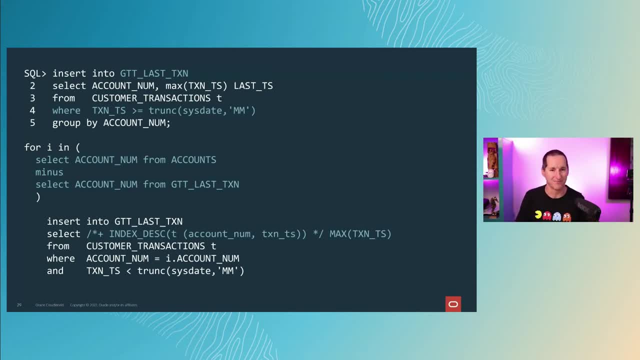 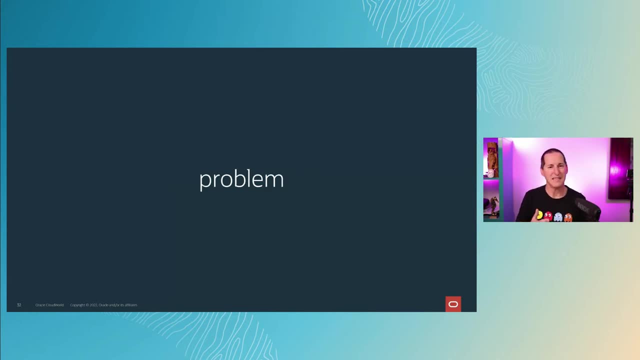 to how it was originally, with all the customers now correctly represented. So we solved the issue, but at the price of a massive jump in complexity. The problem here is being so focused on tuning the SQL, And I get it. As IT practitioners, we love embracing our inner geekiness to solve problems. 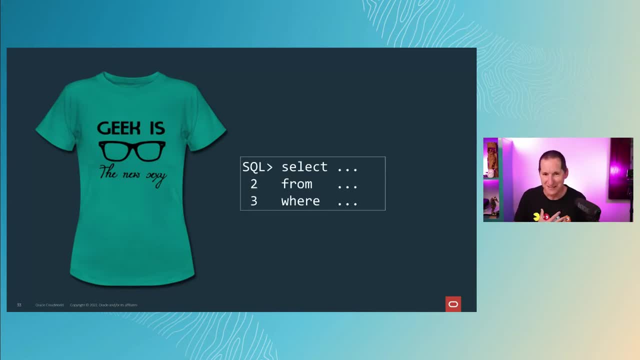 just by looking at code. We all love that ego hit when someone sends an email saying: hey, Connor worked his magic on the code And instead of five hours it now runs in five seconds. Yet we feel like we have superpowers, But rather than adding parallel, adding partitioning, 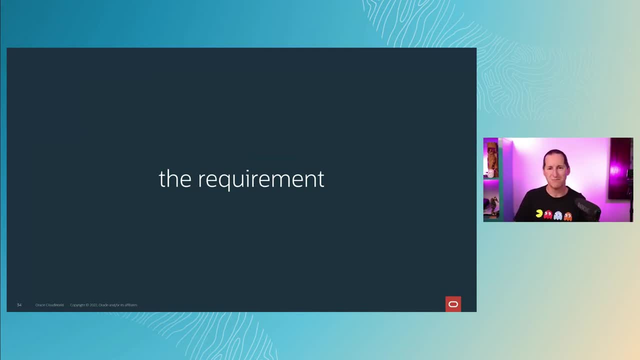 adding, indexing, modifying the SQL. we should have done one simple thing, And that is go back to our business reps and clarify the requirement, Because when we did that, we discovered that the last transaction for all customers was really. we just have an interest in recent 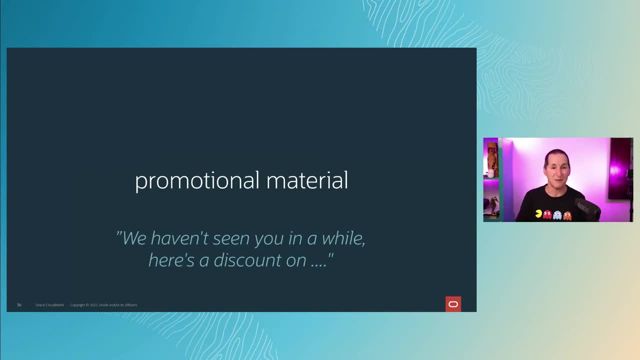 activity for customers, And that's why we're doing this. And that's why we're doing this. They just wanted to know who hadn't been to the website for a while, So we could offer them some sort of carrot, some sort of promo, to come back and hopefully buy more stuff. So what was the 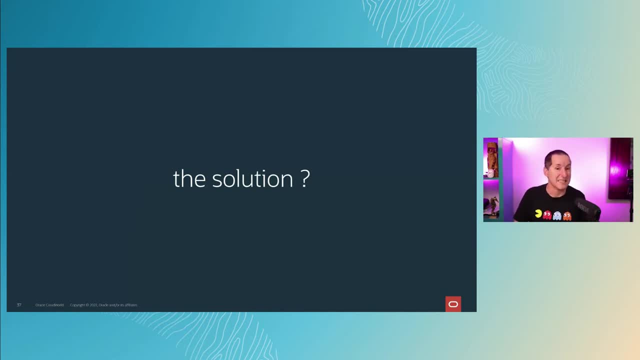 solution we came up with. It wasn't parallelism, It wasn't indexes, It wasn't partitioning. We already had a modification timestamp column on the customer's table which was used to enable optimistic locking. Each time a customer query then updated some data, we would check the 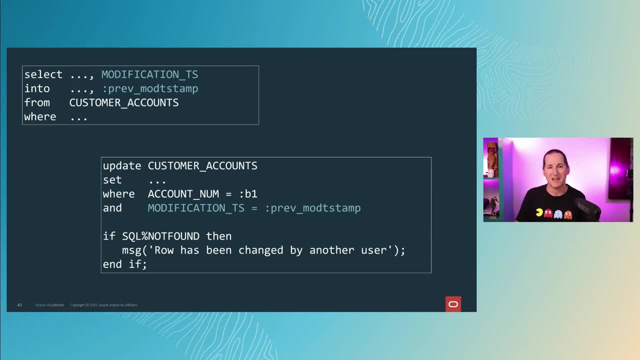 modification timestamp to see if the data was correct, And if so we would check the modification timestamp to see if the data was correct, And if so we would check the current or had become stale. And of course, the modification timestamp is a pretty damn good. 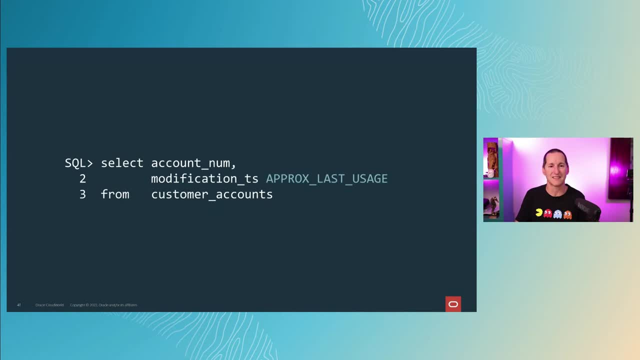 approximation of a customer actually logging on and using their account. They might not have bought something, but they're definitely in our system. So the SQL we ended up writing this report for became select account modification timestamp, which became our approximation for the last usage time for that customer. And that's it. No more performance issues, no more complex. 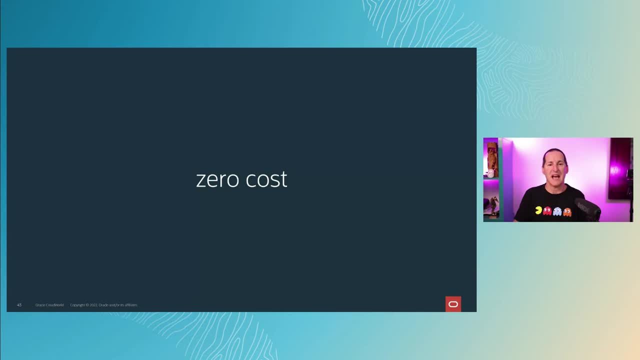 code, no more scanning of those hundreds of millions of rows, And it's zero cost. no partitioning license, no complex code to worry about. But you only spot potential solutions like that if you don't focus on the SQL at hand When solving performance. 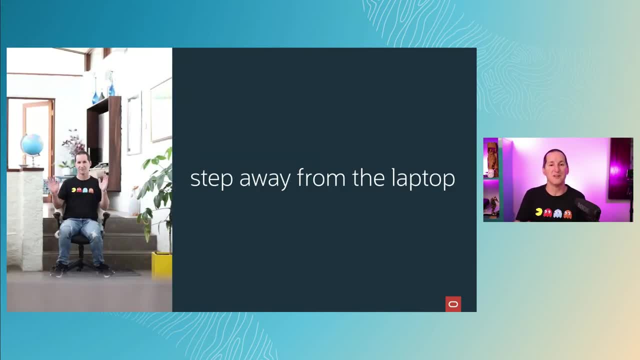 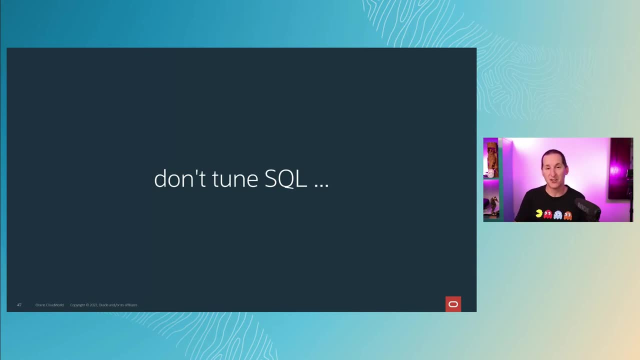 problems. we need to step back from the laptop, step back from the code and look at the bigger picture. So, to reiterate, step one is not the SQL that we're tuning. Now, if we're not SQL tuning, we are doing some tuning, obviously, but it's not this. 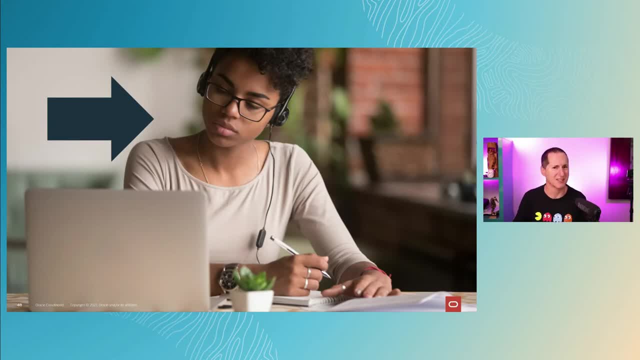 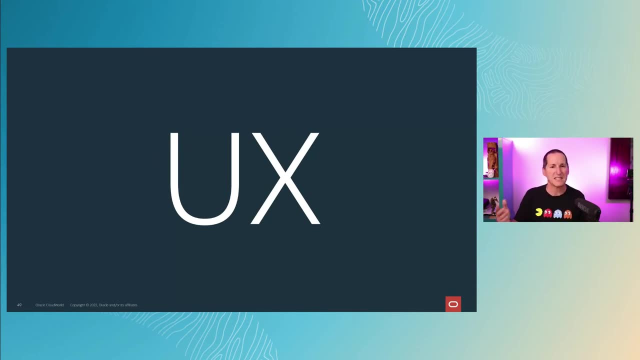 It's this that we're trying to tune. I'm not saying we're tuning the user. What we're tuning is the user experience. Now, this might mean tuning SQL, but it might not be. A SQL that runs for eight hours might be fine if it's only needed in the next day. It can run overnight. 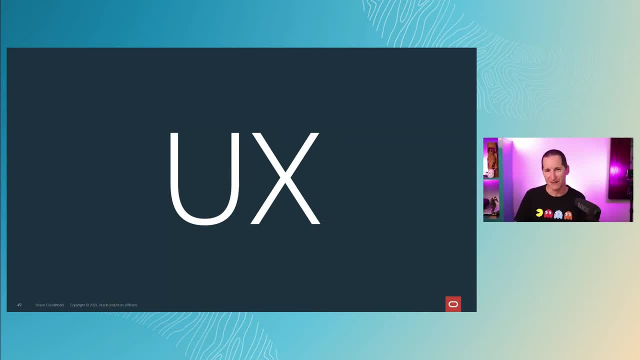 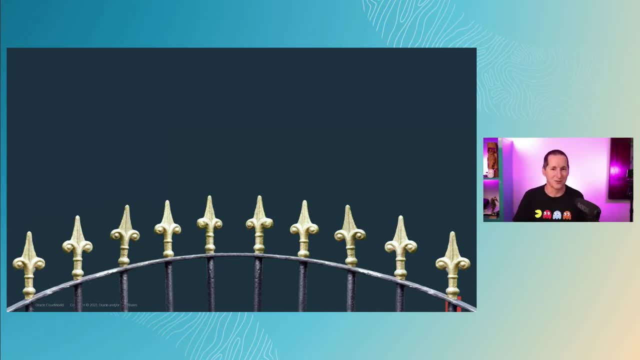 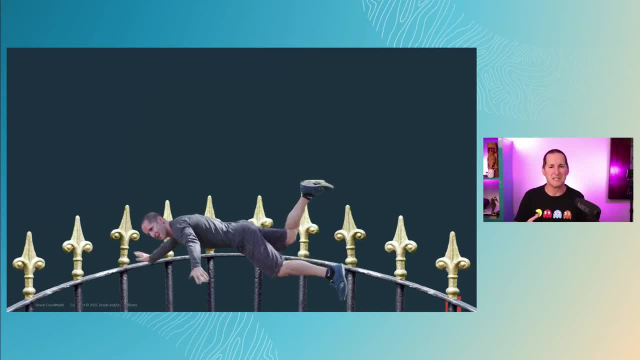 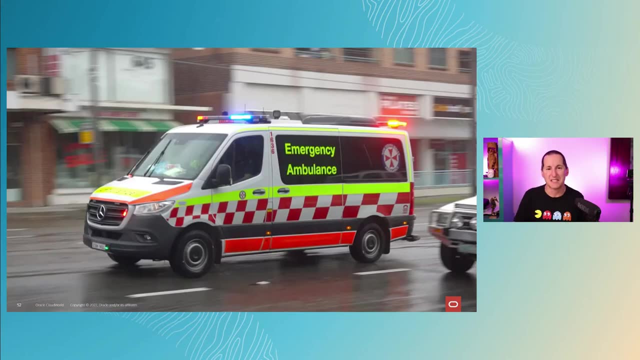 Thankfully my neighbors were there and they called an ambulance, but the paramedics didn't solve anything, They just wrapped a bandage around me and rushed me to hospital. I think of SQL tuning as, like that ambulance, It's not really the cure, It's the triage process. 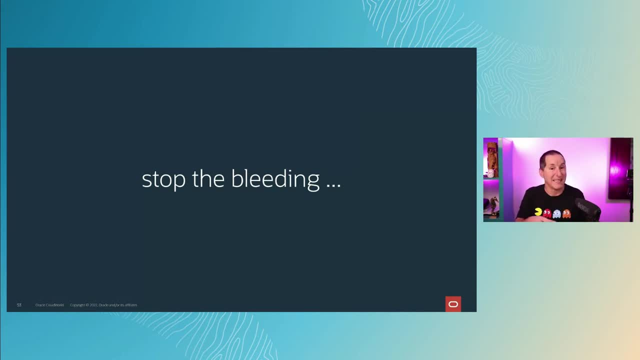 What we're trying to do is just stop the bleeding and stop the pain for the customer. That's what stopping the bleeding is: until we can find a full cure. SQL tuning is just part of the treatment, not the entire treatment of a problem. I'll jump off the soapbox now and continue on. 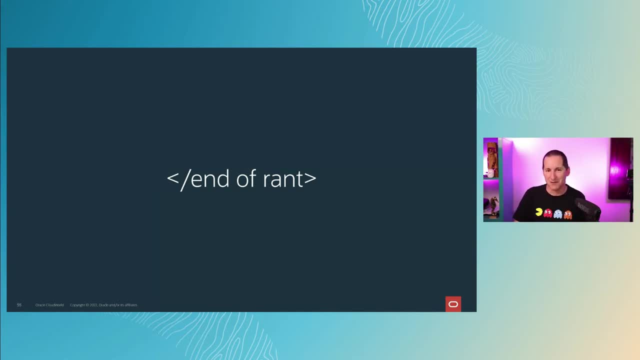 with my ambulance metaphor: Once the ambulance gets to hospital, the doctors are going to work on three things: finding the cause of the problem, then treating that problem and then working toward a cure. Let's apply those three phases to the act of solving a SQL tuning problem. Step two: 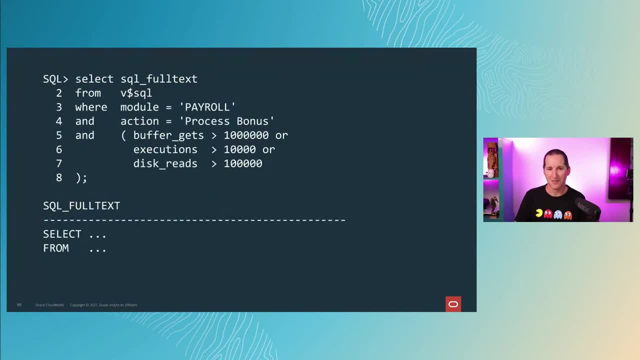 is to solve the problem. Let's apply those three phases to the act of solving a SQL tuning problem. Step three is finding problematic SQL in your system. Anyone involved with SQL tuning typically has a query like this one. in your toolkit, You narrow down your focus to a particular 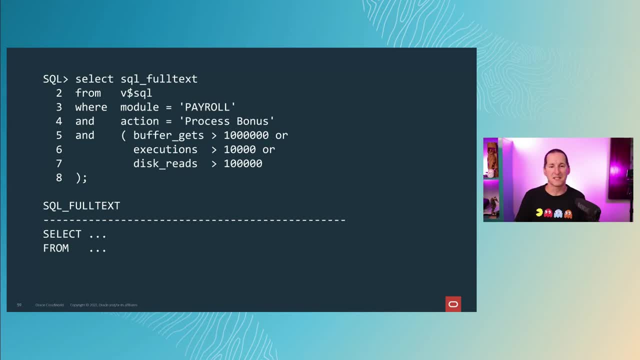 part of the application, such as payroll, and then you look for SQLs that are smashing. either the CPU buffer gets running too many times or hurting your IO subsystem. This is a bad place to look for SQL tuning because of latching. Latching is the way we control access to memory. 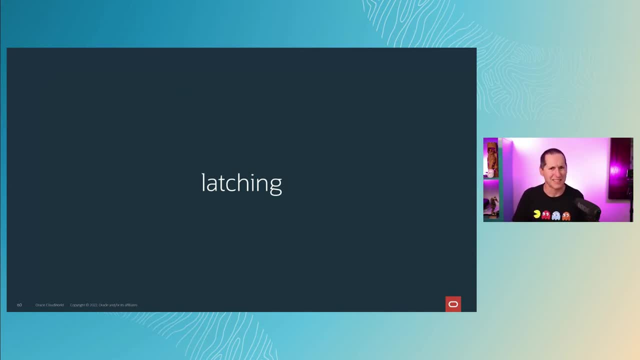 structures inside the Oracle database. This is a bad place to look for SQL tuning because of latching. Latching is the way we control access to memory structures inside the Oracle database. It's a bit like using a public toilet: You latch the door to make sure that you're the only person. 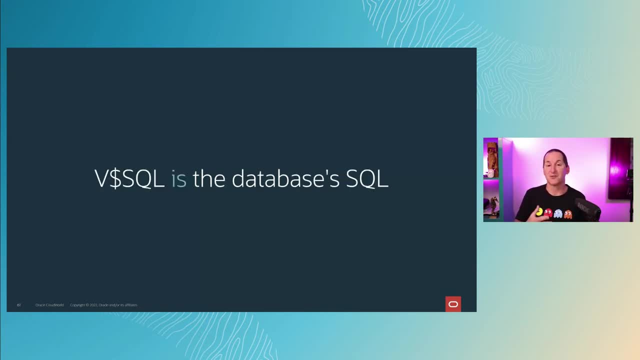 using it at the same time. V$SQL is a direct view into the memory structures of the running SQL in your system In the database. if you access that structure then you need latches to control access to that memory. But if you've grabbed a latch to look at V$SQL then you're hurting concurrent. 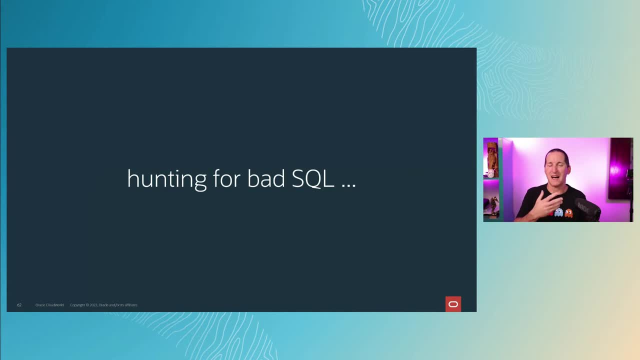 access to your system. What that means is you're hunting for SQLs that are bad, with a SQL that's probably going to hurt your system. That's not a smart way. There's nothing worse than when you get called in to help with a SQL tuning problem and everyone noticing 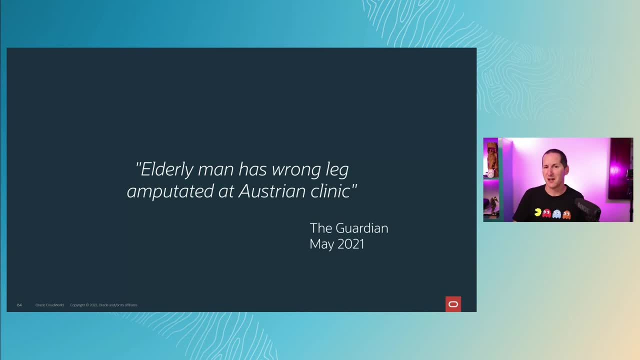 that the moment you've logged on to your system is everything is actually getting slower, not better. That's not a great way. It's like this story here. Make sure you don't pick the wrong leg. There is a better option than using V$SQL. 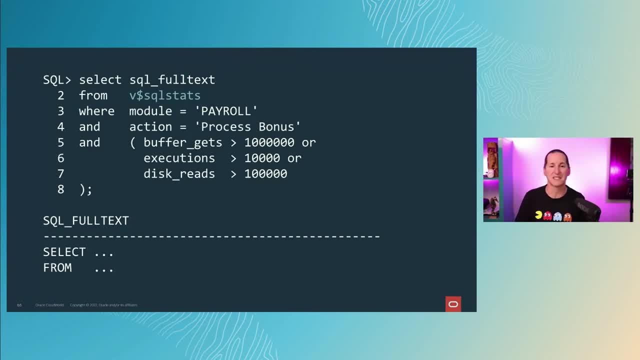 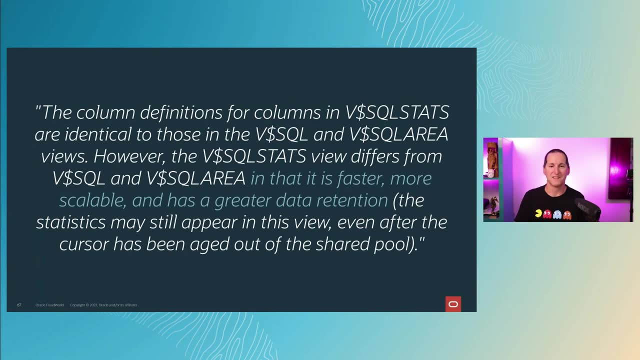 Since as long ago as 10G, there's a partner view to V$SQL called V$SQL Stats. Rather than having me explain why it's better, let me grab that reference straight out of the documentation. The column definitions of V$SQL Stats are identical to V$SQL, However, it is faster. 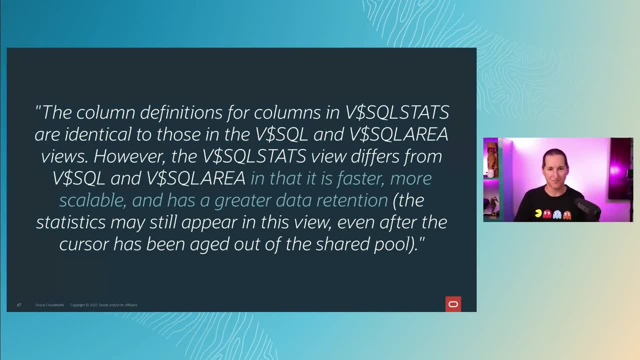 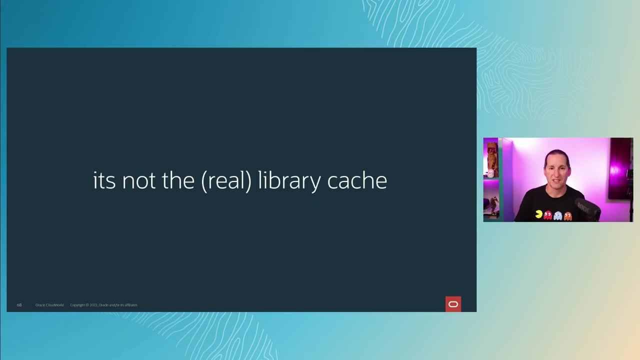 more scalable and has greater data retention. It's generally a better option And because it's a separate memory structure from the real library cache, which is V$SQL, it's also designed that it can be queried quite aggressively without using latches. It's not the real library cache. So now you're using the V$SQL Stats, which is V$SQL Stats, which is V$SQL Stats. So now you're using the V$SQL Stats, which is V$SQL Stats. So now you're using the V$SQL Stats. So now you're. 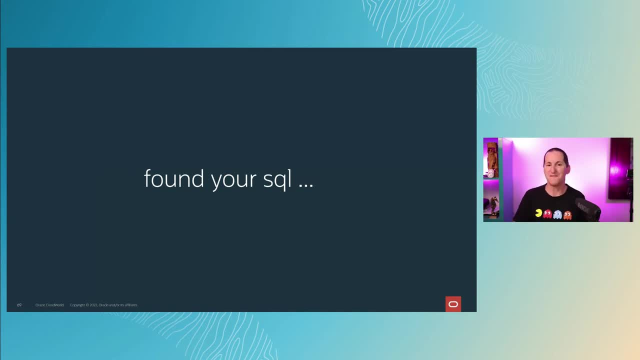 using V$SQL Stats to find your problematic SQL. Once you've found it, it's time to move on to step three. Step three is treating the symptoms. Let's assume this is the query we need to improve. We've got a table of vehicles with manufacturer details, such as make and models, And I've got 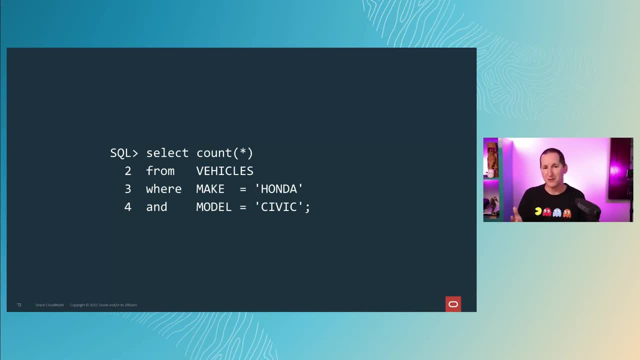 a simple SQL here looking for Honda Civics. But even though it looks simple, simple SQLs can be deceiving. No matter how simple a query looks, the first step is to determine whether it is actually as simple as it really appears. Here's a slightly different example. I'm querying: 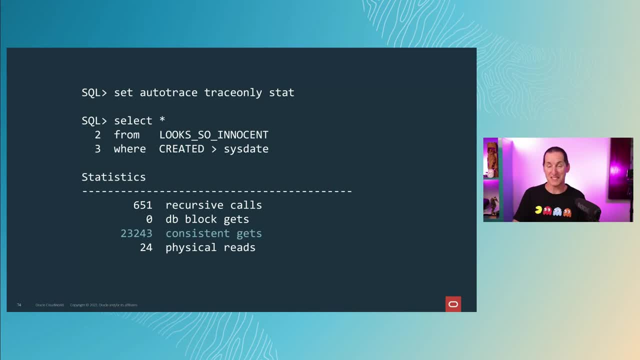 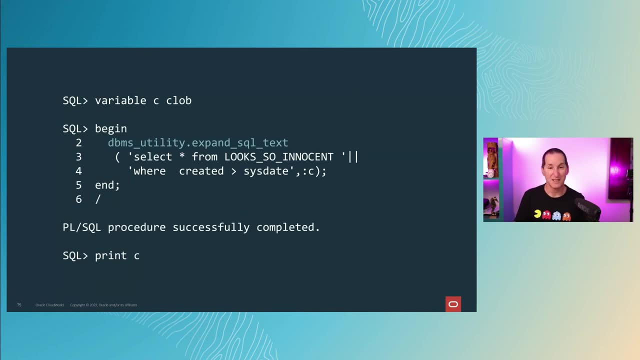 something which I've called looks so innocent, But you can see from the consistent gets below, it's actually quite an expensive query. Inside the DBMS utility package we have a cool routine called expand SQL text, which expands out all the components of a query to discover what 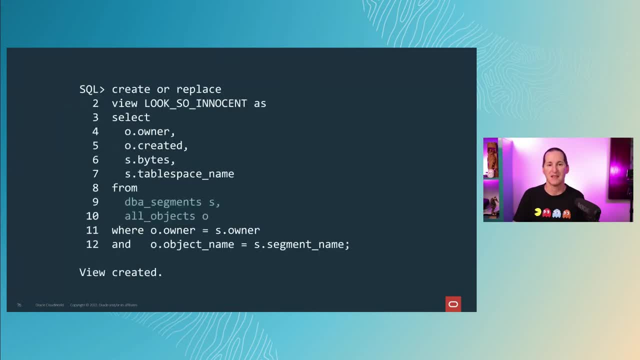 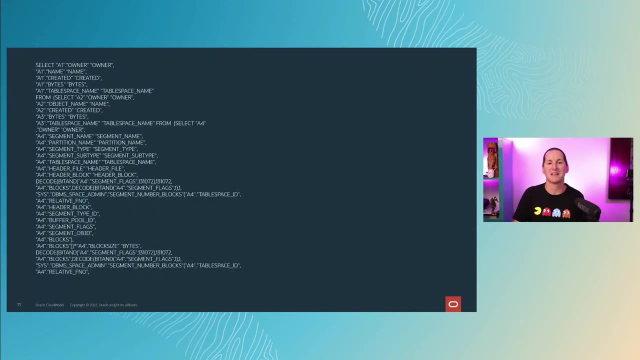 the database will really see when it runs. your SQL, In this case, looks so innocent, is a view that joins DBA segments and all objects. They're both dictionary views as well, So it's a view of views. When we expand the SQL text fully using DBMS utility, we get this, But we're not done yet. 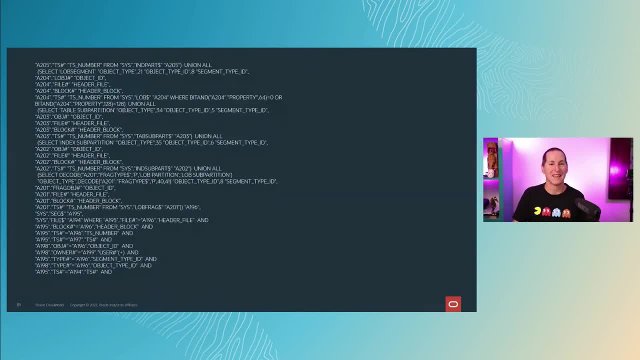 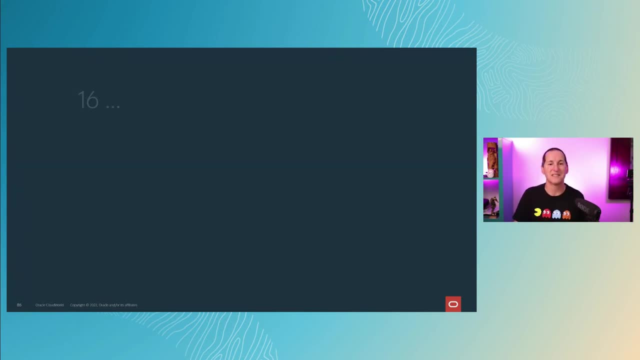 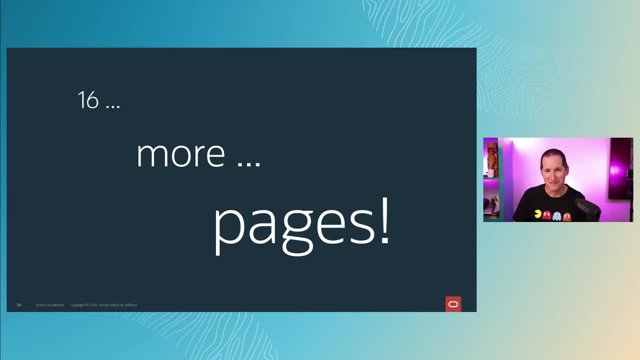 checking. It's always worth checking. It's always worth checking. A short SQL in your app might be a monster for your database to handle. Once you've found the real SQL, the next step is where you want to check before tuning it is: does the SQL statement actually make sense? I've lost track of the number of times a slow SQL 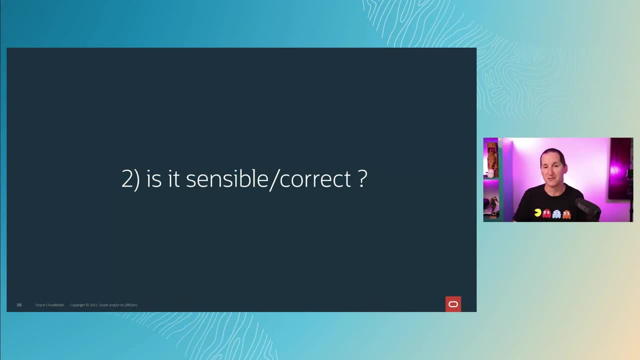 is simply slow because it is not actually correct. It doesn't meet the actual requirement. For example, here we have a query against the employee and department table, But something's missing. The join condition was forgotten, You might be thinking. but 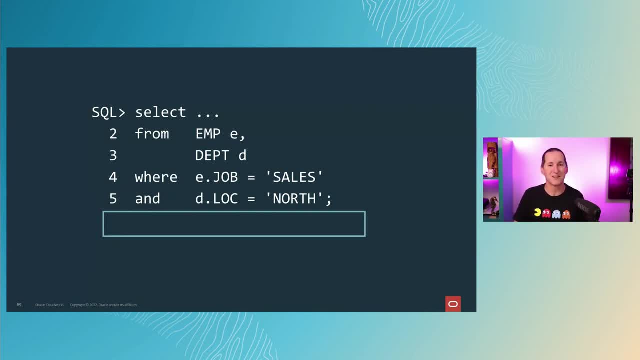 this would then return too many rows and it would be obviously wrong. But people often solve this by simply adding a distinct and they think, yep, everything's fine, But that's going to run very slowly because of the Cartesian product, Or similarly, this query looks fine until you. 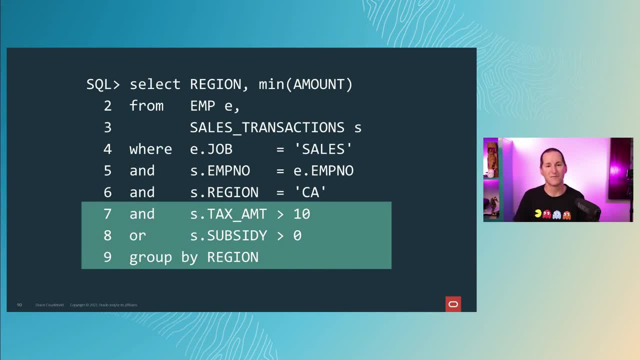 realize that AND takes precedence over OR, which means in this query we get all the rows that match the employee condition or the region condition or the tax condition, or every single row for which a subset is greater than zero. We needed to have some brackets in there. a. 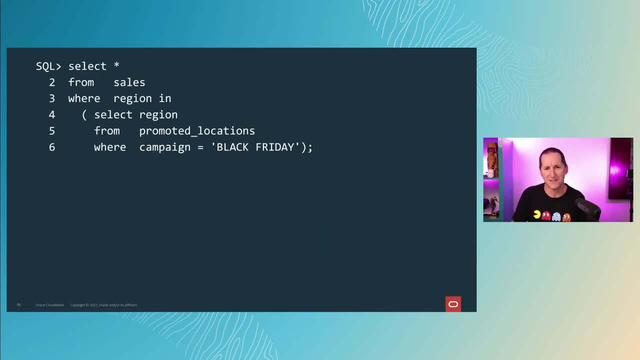 round our OR condition, Or this slightly less obvious one. This query looks fine, but you can see that there's actually no column called region in the subquery table. This query does not crash, though, with an error, because region is actually taken from the parent table and becomes an always. 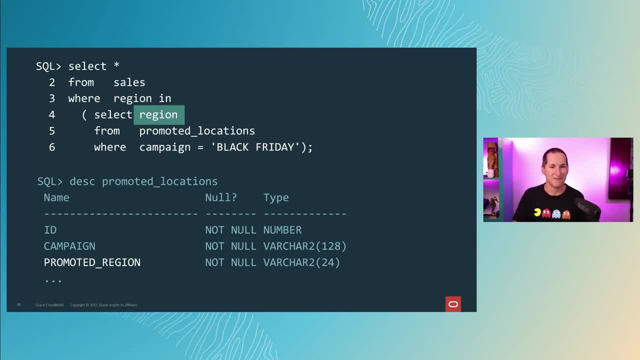 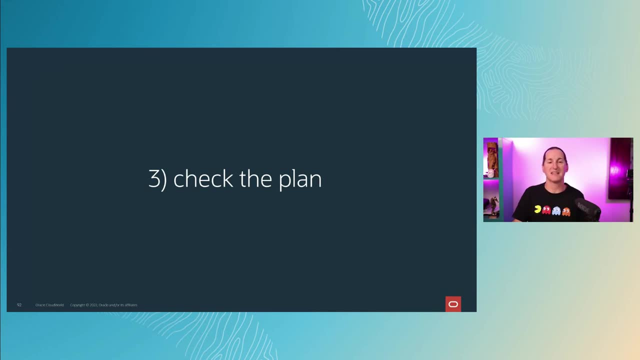 true subquery. This is another reason to always alias and reference your columns If the SQL is indeed logically correct. the next step is to check the execution plan to see how the optimizer should run the query. We're trying to see here if the optimizer made a bad decision somewhere in. 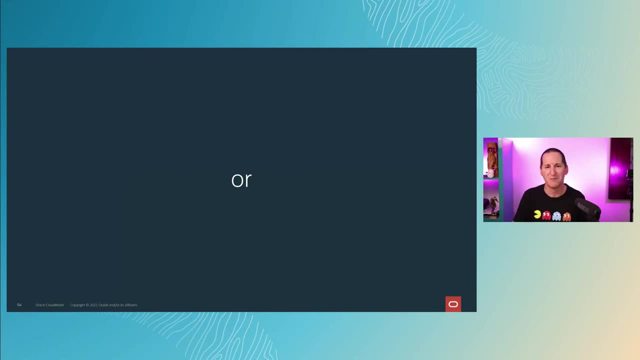 its process, OR- and I wanted to include this- OR, because we often forget about it. it's quite possible that a slow SQL simply can't be made to run faster. Sometimes SQL tuning is just talking to the customer, saying, look, you're trawling through 20 years of data to get a single grand. 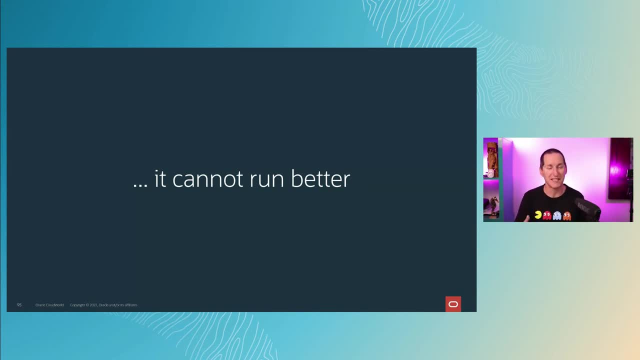 total. It's a lot of work for the database to do. Sometimes just that explanation is all it needs to convince the customer to run the query. We're trying to see here if the optimizer made a bad decision somewhere in its process Or- and I wanted to include this- OR, because we often forget about. it. it's quite possible that a slow SQL simply can't be made to run faster. Sometimes SQL tuning is just talking to the customer saying, look, you're trawling through 20 years of data to get a single grand total. It's a lot of work for the database to do. Sometimes SQL tuning is all it needs to. convince the customer to run the query We're trying to see here. if the optimizer made a bad decision somewhere in its process, Or- and I wanted to include this- OR because we often forget about it, it's quite possible that a slow SQL tuning is all it needs to convince the customer to run the 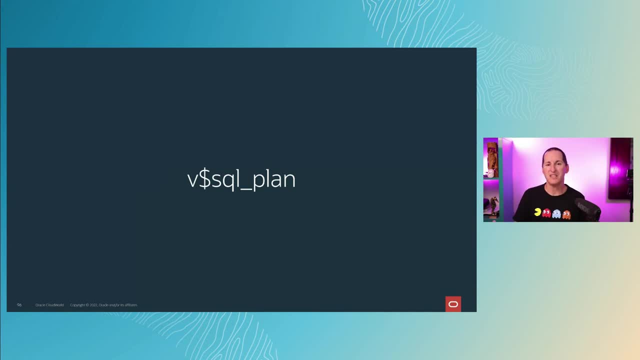 query We're trying to see here if the optimizer made a bad decision somewhere in its process. But back to the optimizer. The way we check an optimizer decision is to either look in VLLS SQL plan or we can just use DBMSX plan display cursor, which will interrogate VLLS SQL plan for us. and 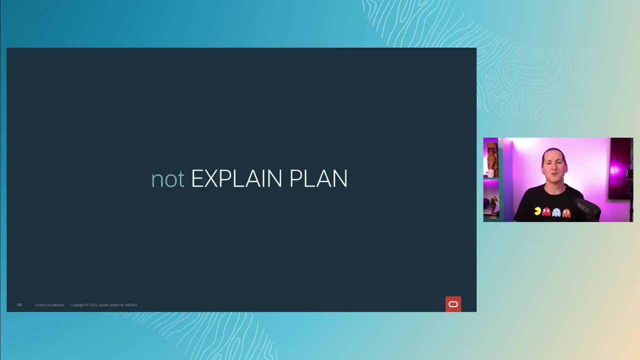 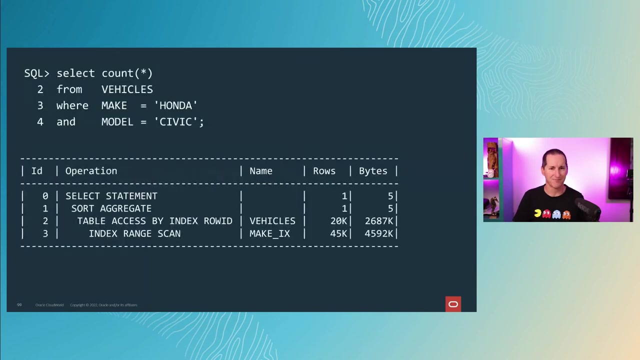 give us a nicely formatted execution plan, But one thing that we should not use is explain plan command. Don't get me wrong. it's a useful tool for seeing, perhaps roughly, what the optimizer is going to do, But let me give you an example of why it's not as good as many people make out. Here's the: 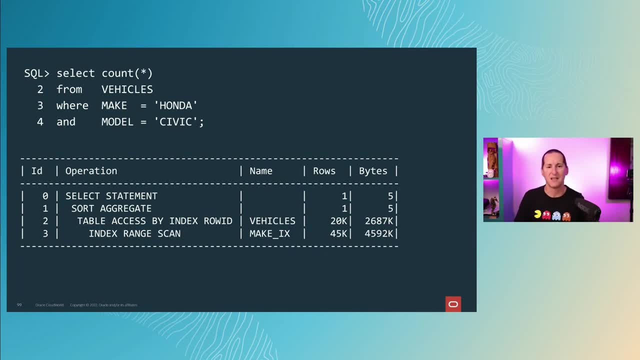 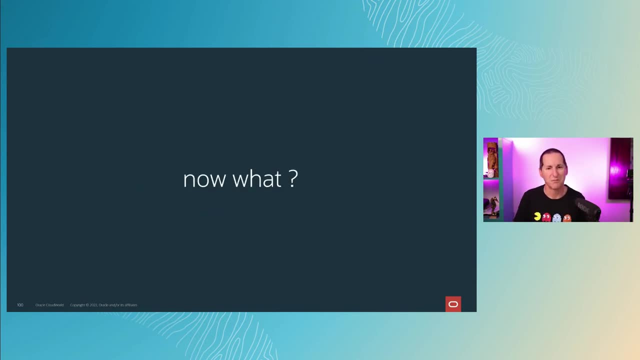 execution plan for my query against the vehicles table that I showed before. We can see it's using the index, presumably on the make column. My question to you is now: what Is that a good plan? Is it a bad plan? We can't tell just by looking at the explain plan. It doesn't really reveal. 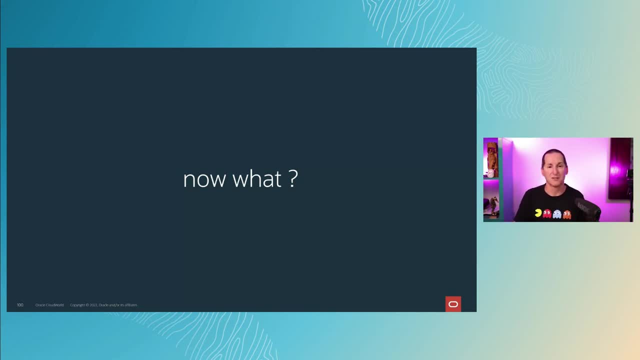 enough information about whether a query is going to run good or not. When a doctor needs more information, they'll say: where does it hurt? They'll poke you and prod you and stuff. And we can do the same for SQL statement. We can drill into whereabouts in the plan, the optimizer, either. 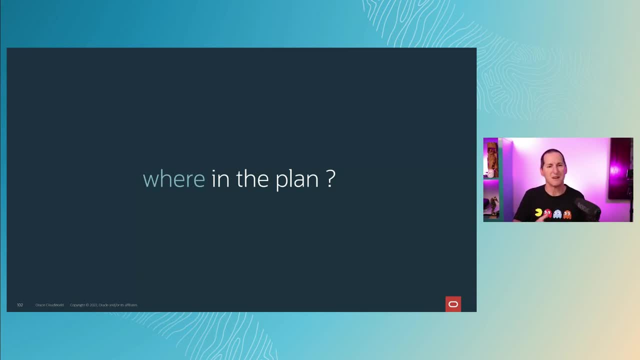 made a good decision or perhaps lost its way. The optimizer is a lot like a person. Let me explain. For human beings, cardinality is a really important thing. Now I imagine you don't use the word cardinality in everyday life, So let me explain what I mean by cardinality. Sometimes I'll pop. 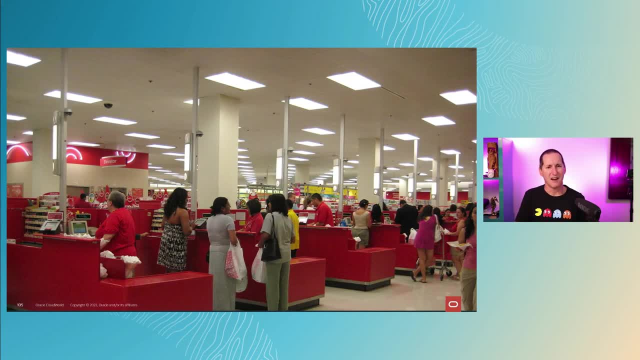 down the shop to grab a few things. When I get to the checkout, I don't just go to the first checkout, I look along the whole line of aisles and I look for the best one And I scoot down to that one. 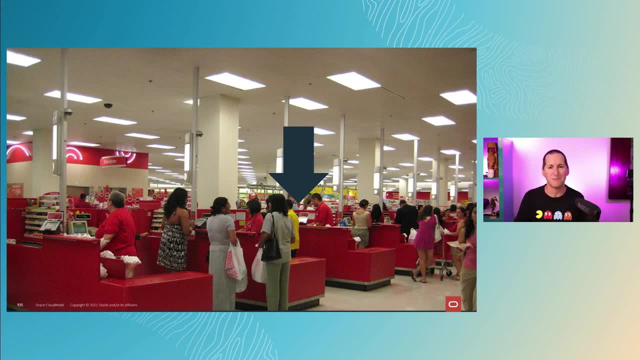 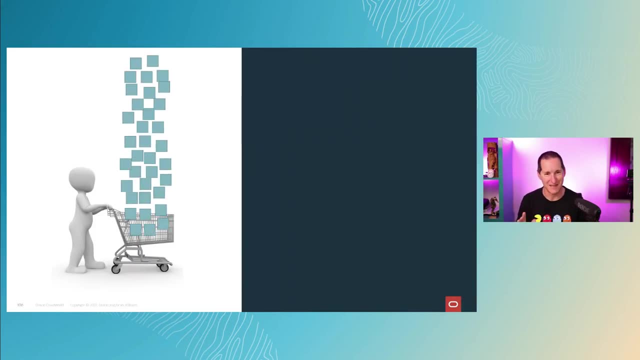 In fact there's one guy just in yellow. there There's only one guy. I'll queue up behind him, But sometimes I'll get there, and that one guy has got like the shopping trolley from hell. Yeah, there's a million small things that he's going to go through the checkout with And I'm 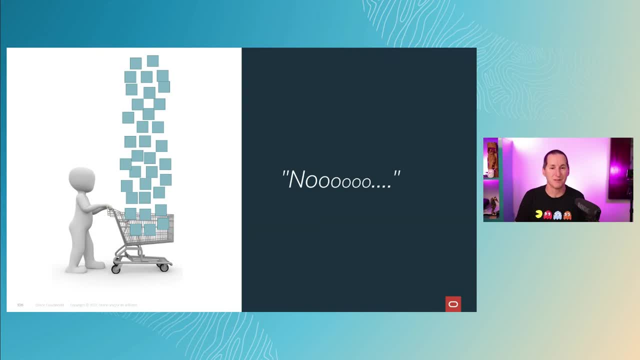 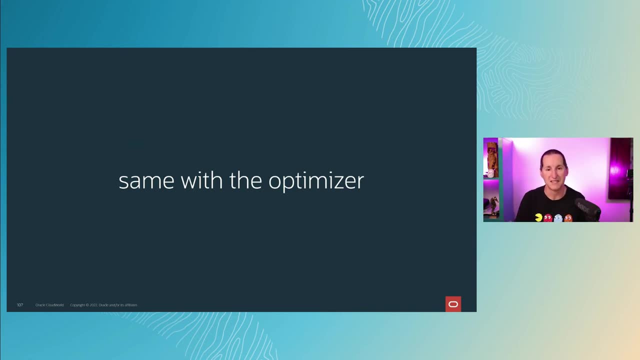 like, oh no, I'm going to be here forever And that's a problem. It's the same with the optimizer: It made a prediction or an estimate for each step in the plan that it thinks is best. If the actual results during runtime don't match that estimate. 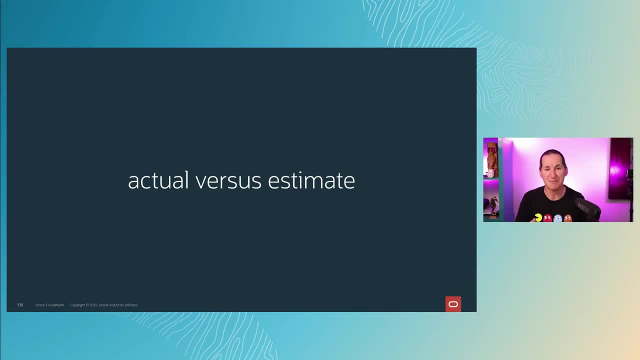 it's likely to be a bad plan. If it matches the estimate, it's likely to be a good plan. It's much like me going to the supermarket. If the guy in front of me didn't have many items, because that was my prediction, then I'm going to have a good experience And we can do this with the gather. 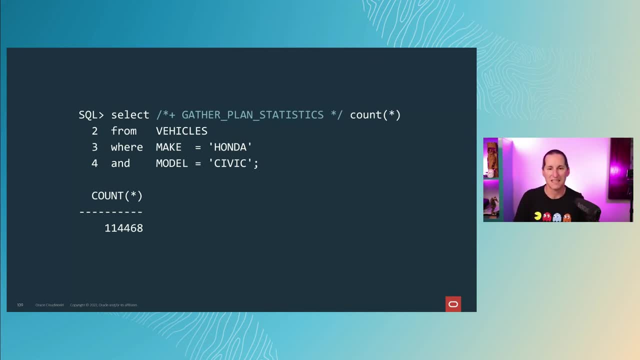 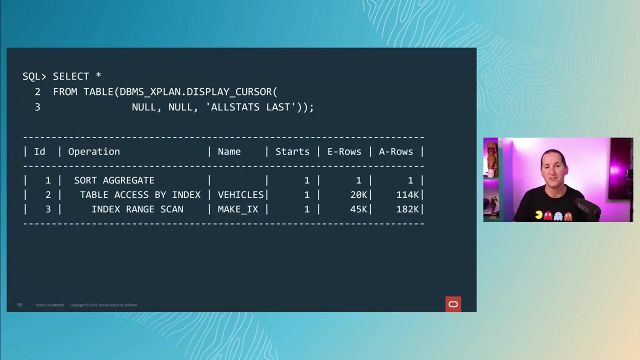 plan statistics hint with our SQL. When we run a statement with this hint, the database will record both the estimated plan by the optimizer and the actual runtime statistics as well. In our example, we can see that there are about 114,000 Honda Civics in our table Using DBMSX plan. we can see that the same 114,000 Honda Civics test that's been test as if we went beyond point 21. its Tricolor model shows that there are a evaluation change in the product's return to its depreciation rate. Aren't we ever willing to? Jordi toddy can give you a look and hear about the difference between a project, nor an. 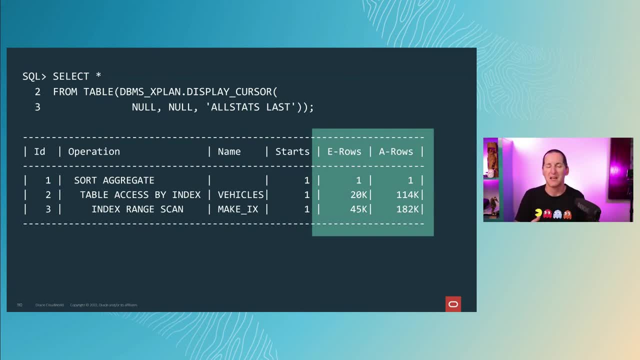 14,000 number in the A for actual row columns, But the optimist estimated that in the E column that there was actually only going to be 45,000 Hondas- that's the make index- of which only 25,000. 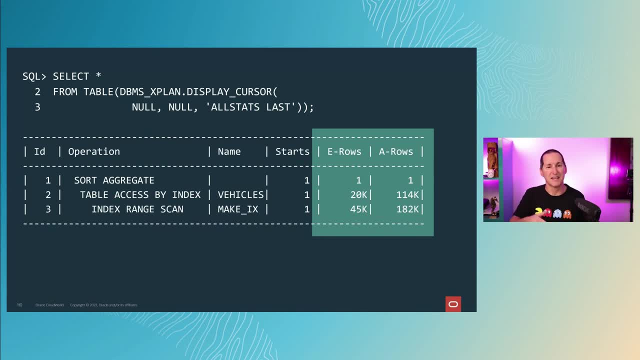 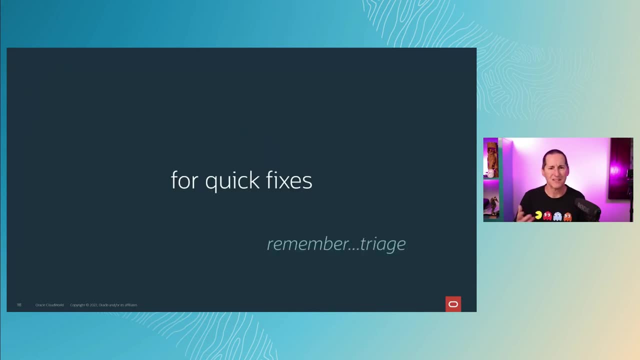 were going to be Honda Civics, So the estimate didn't really match the actual result. So, just like the supermarket, the result probably is not the optimal one, Putting our triage hat on again. sometimes we are just looking for quick fixes in order to get this SQL statement running. 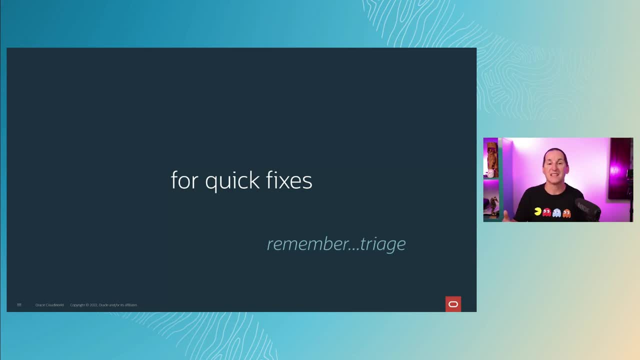 The optimizer chose an index because it expected far less rows than actually came out of the query. Perhaps a full table scan would have been a better option here, So we can use a hint for that. We've told the optimizer that we know better In this case. I know Honda Civics sell really well. 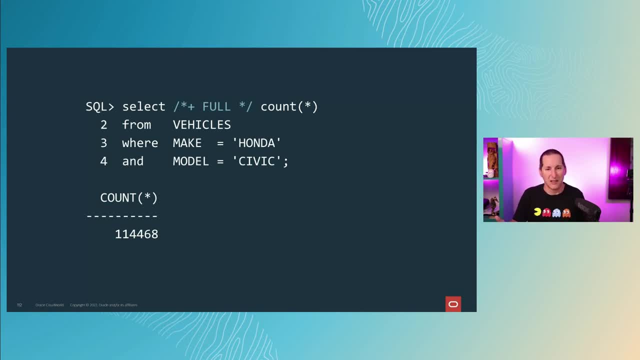 where I live, There's 114,000 of them, So there's always going to be a lot. But I need to stress here: It works for this particular example. But when it comes to hints, I'm not saying that hints are going to be a good idea. I'm not saying that hints are going to be a good idea. I'm not saying 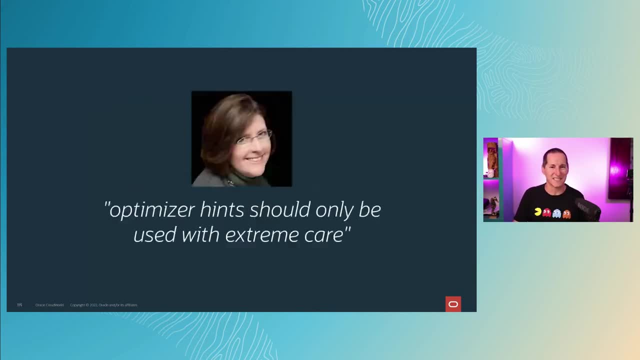 that hints are the solution. As my good friend Maria Colgan often says, optimizer hints should only be used with extreme care. I often phrase this as the optimal number of hints in any application is zero. But remember, this is triage. We're looking for quick fixes until we can move. 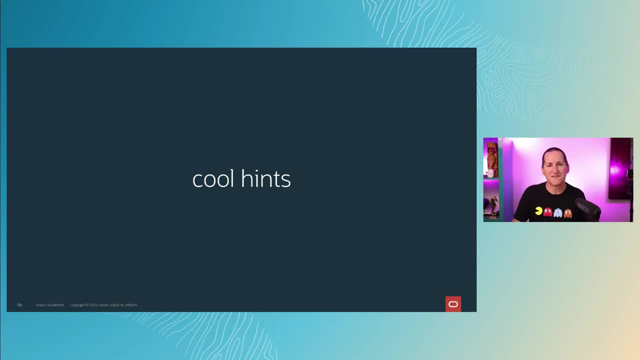 toward coming up with a proper cure. If you're using hints for triage, try limit yourself to what I call the cool hints. Some examples of what I call cool hints are these ones. Each one is typically trying to optimize the results of the query. So if you're using hints for triage, 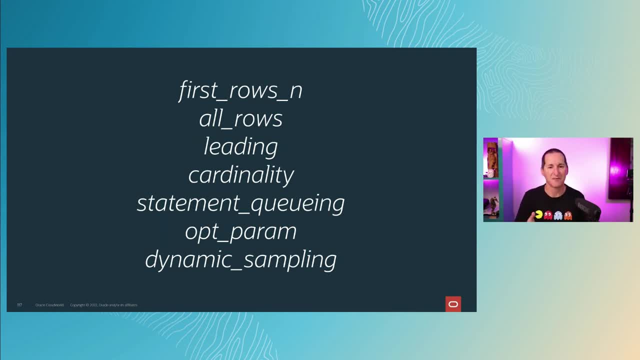 you might want to offer the optimizer more information about the query. I just want the first rows, or this is the best table to start with. That's the leading hint. These are hints that are trying to assist the optimizer with its decision making process because we might know more. 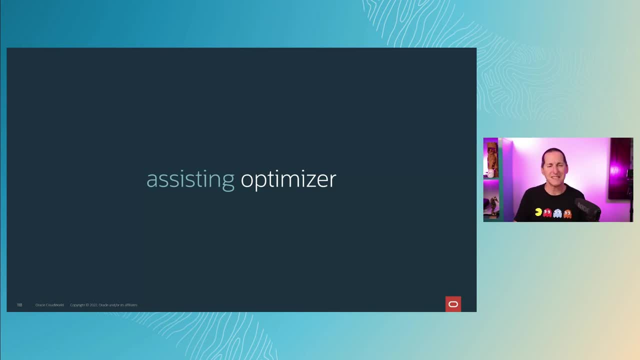 about the data than the optimizer does. Conversely, there are what I call the dangerous hints. The list of hints of these hints is pretty simple. It's everything else. I'm not saying you should not use them, But ideally these are used. 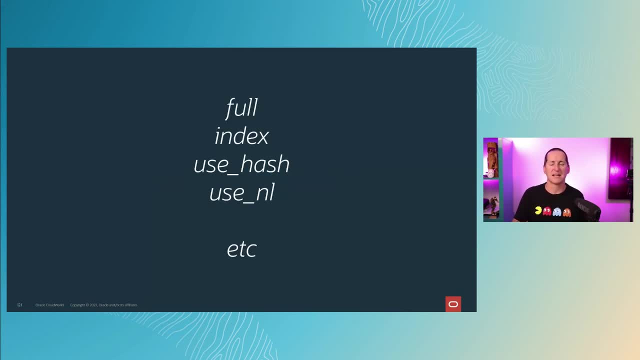 If we look at some of the common ones that are used, like full or index or force or join method, then, in effect, you're choosing to suppress the optimizer rather than assist it. You're limiting the number of decisions it's allowed to make. You're taking away options from its disposal. 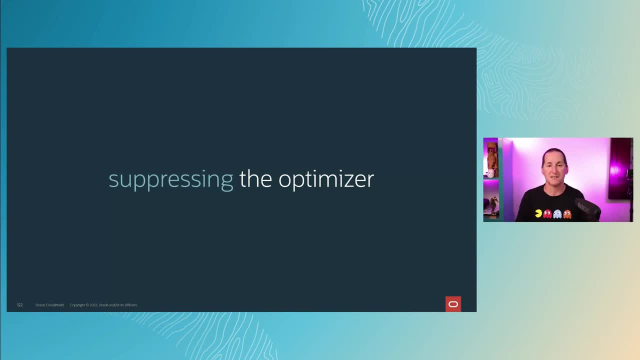 Now, as data changes over time, this suppression can lead to more performance errors. Maybe a plan should change over time, but you've told the optimizer it's not allowed to. As I said, hints are just a temporary fix. They're triage. 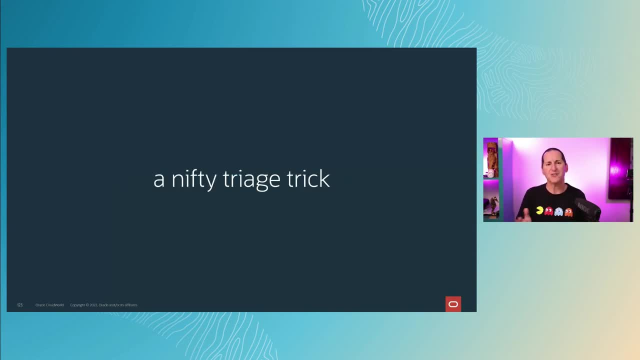 we're trying to stop the bleeding. If you do use a hint as a temporary fix, here's a nifty trick to ensure that your fix is reasonably robust. Once you have the execution plan you need, by adding a few hints, use the plus outline format extension in DBMSX plan. 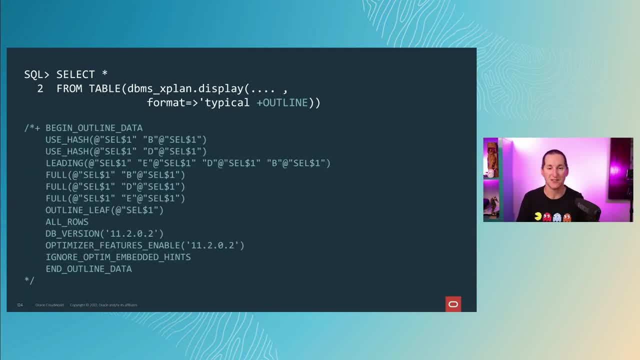 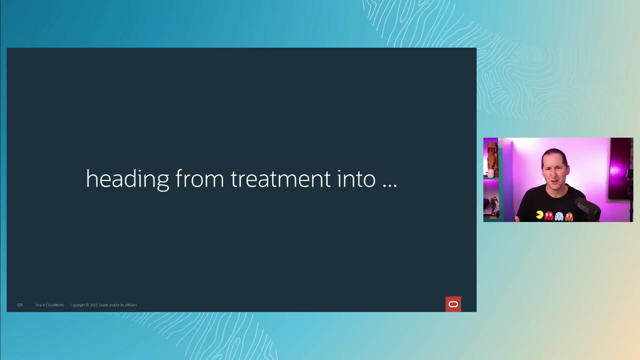 This will output a comprehensive set of hints that you can use to lock the plan you want into place. It's formatted in the correct hint syntax, so you simply just paste it into your SQL code and you're good to go. So now I've done some initial treatment, a bit of triage, Just like the hospital, I like to come up. 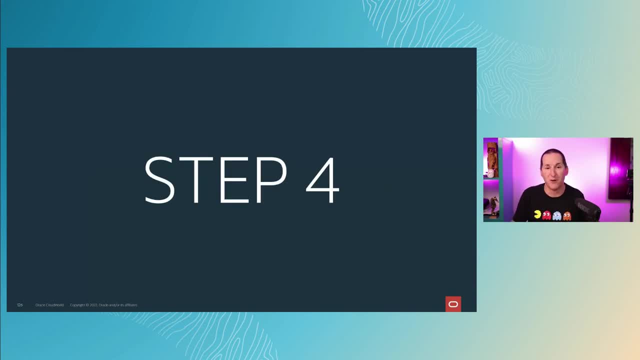 with something which is more permanent. It's time for step four. I'm looking for the way that I can send my patient home fully cured. If you break an arm, you'll get sent home in a splint. It's the same with a problem SQL statement. Maybe you need not to fix the SQL, but just the periphery in. 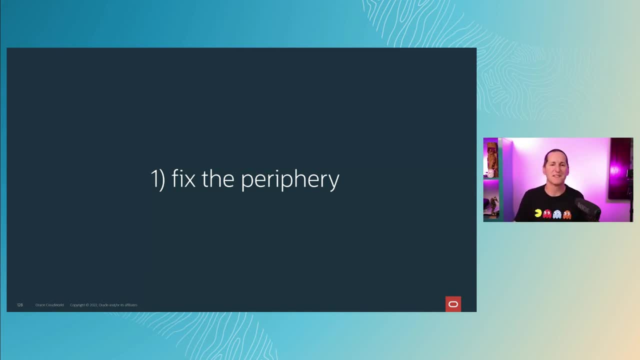 order to let the SQL heal itself. naturally, This often involves adding or removing indexes, and the key thing here is to make sure that the SQL is in the right place. If the SQL is in the wrong place, the key thing here is to make sure that you add or remove them safely. One of my favorite quotes: 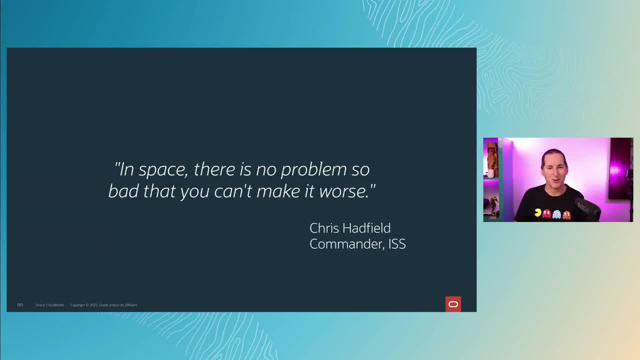 about tackling problems comes from NASA, namely in space. there is no problem so bad that you can't make it worse, And it's the same with the database. Adding or removing indexes is a high risk option because it could change the entire performance profile of many other SQL statements in your 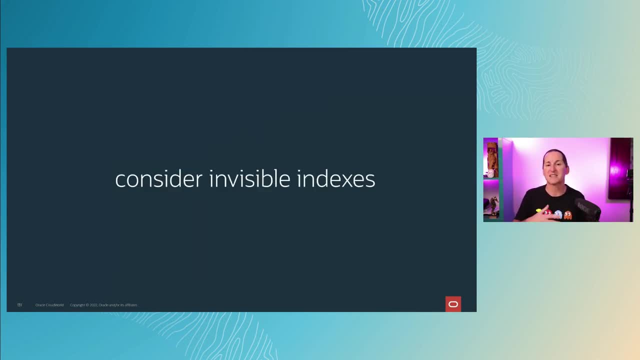 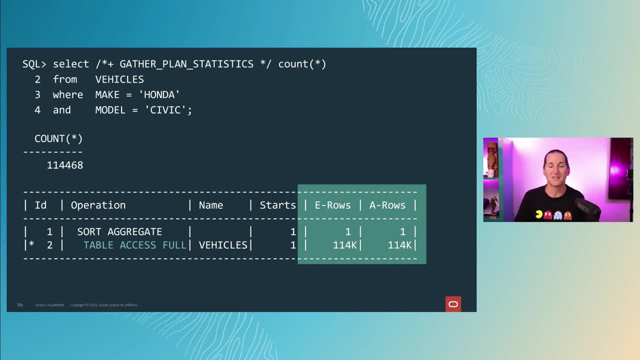 using the invisible indexes To drop an index. make it invisible. If you're altering indexes, then consider using the invisible indexes To drop an index. make it invisible. If you're altering indexes, then consider using the invisible indexes To drop an index. make it invisible. If you're altering indexes, then consider. 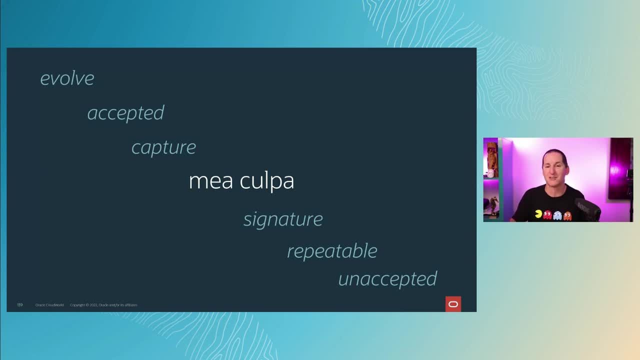 page and shout SQL tuning. So I can understand people didn't really adopt it aggressively. But in reality the feature is very simple And if we strip off the terminology, it offers three things we strive for, namely: I like this plan, so please use it. I don't like this plan, so you're not. 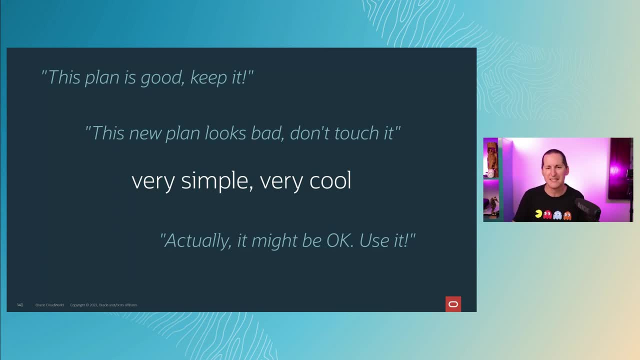 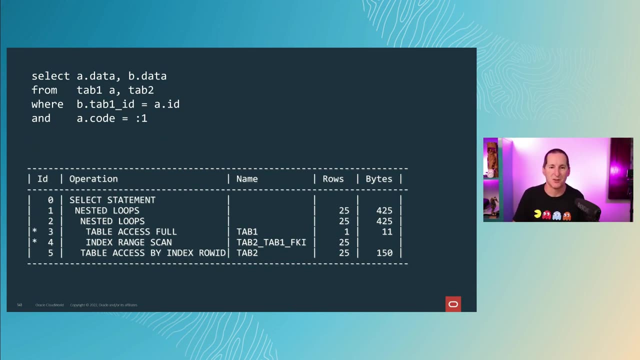 allowed to use it. Or maybe over time that bad plan has become a good plan. So let's have another look. Let's look at it in action. Here's a standard SQL statement And here's the plan. the optimizer chose to run it with Nothing out of the ordinary there In SPM technology, we call that an accepted 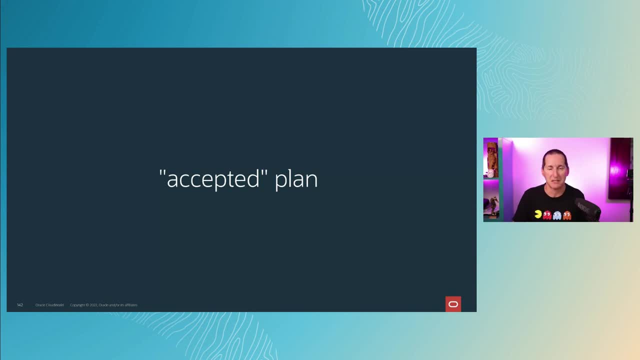 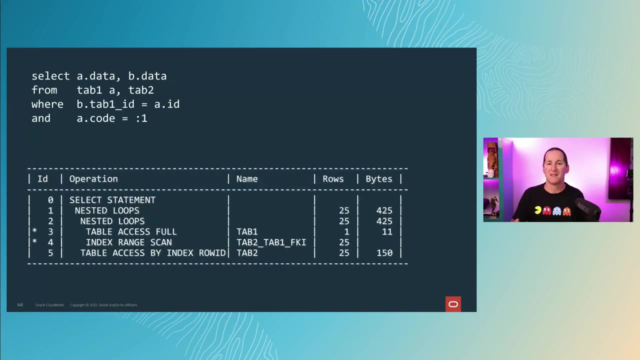 plan. This is a plan that can be used by this particular SQL. If you're not using SPM at all, then obviously every plan is an accepted plan, But when SPM is in play, then only plans that are accepted are allowed to be used. As we know, plans can change over time. the stats get updated. 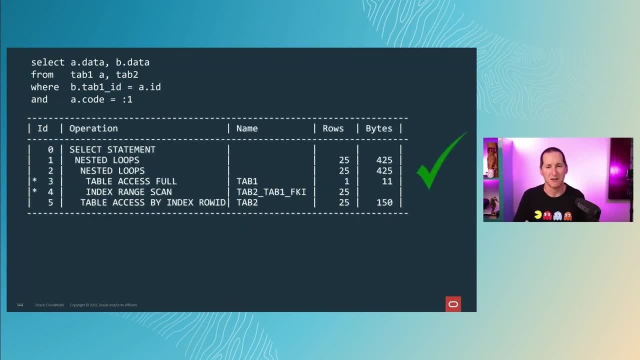 the data changes, etc. So each time we pass this SQL we might get the same plan or we might get a new plan, But with SPM, because we have an accepted plan, this new plan is not accepted by default, Even though we passed it and the optimizer said: yes, it's the new plan. 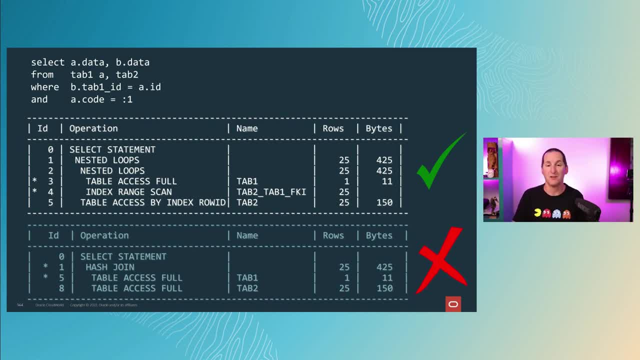 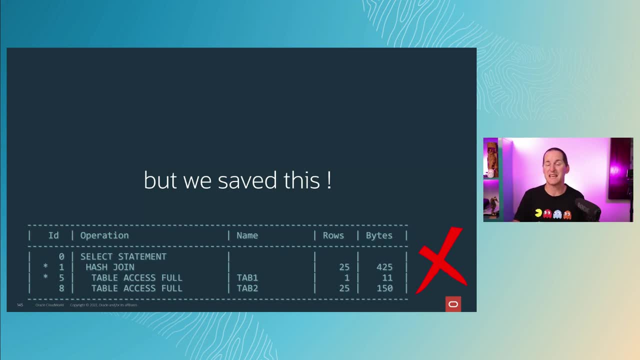 this is the one I want to use. it will not use it. It will only use the accepted plan. The cool thing with SPM is we don't just throw it away that plan that wasn't used. we save it Because this is the plan the optimizer now thought was the best plan, even though we didn't use it. 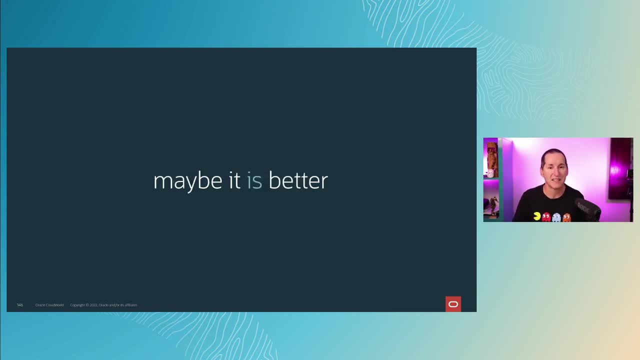 And maybe over time it is better. Maybe the optimizer was right, Maybe the data has changed enough for that new plan to be the best plan. SPM doesn't mean I can only have one accepted plan. I can tell SPM to evolve a plan. 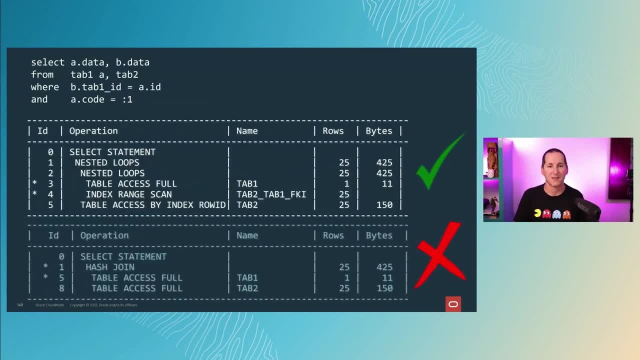 This lets me tell the optimizer this new plan is also accepted. The new plan which we originally blocked from usage now becomes an accepted plan as well. Each time we pass this query, the optimizer can come up with either of those plans and they'll be allowed to be used If it comes up with a third. 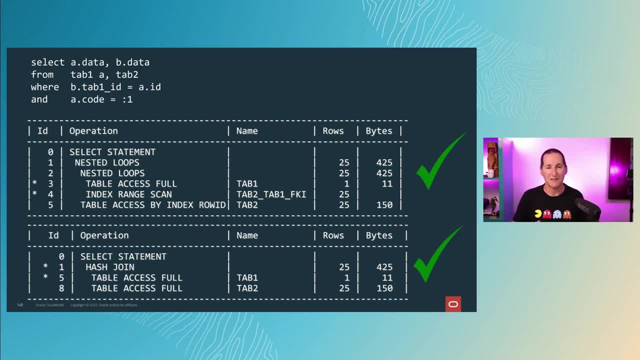 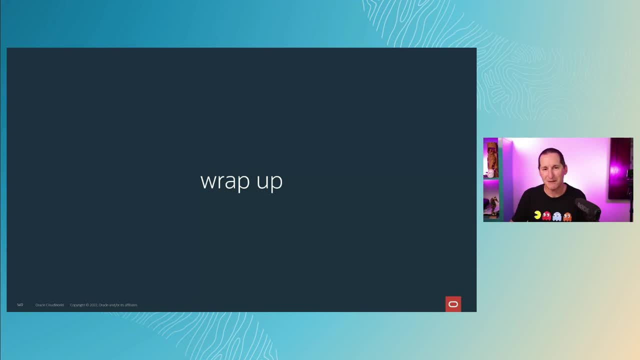 brand new plan. it will be accepted. It won't be allowed until we go look at it. We have this very total control method of choosing which plans we want to allow the optimizer to pick. Let's wrap up this session on SQL tuning by reiterating: If you're tuning just SQL, then you're perhaps focusing on the wrong thing.